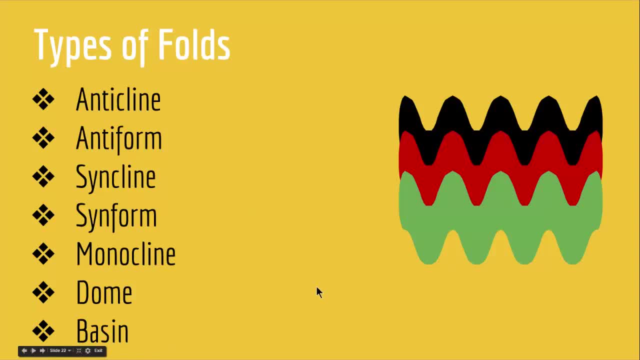 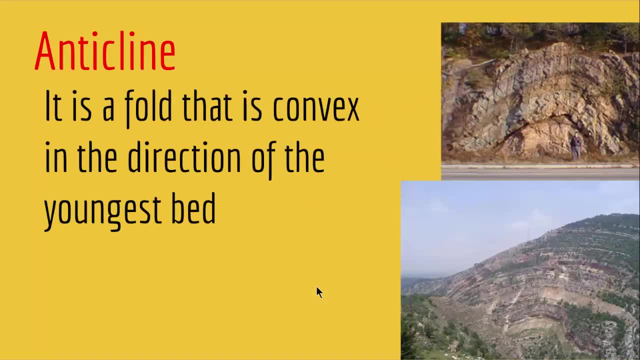 All these are types of folds, So let's look at each of them in more detail. The first one: an anticline. What is an anticline? Well, an anticline is a fold that is convex in the direction of the youngest bit. If you have bits stacked on each other and you bend them, or you. 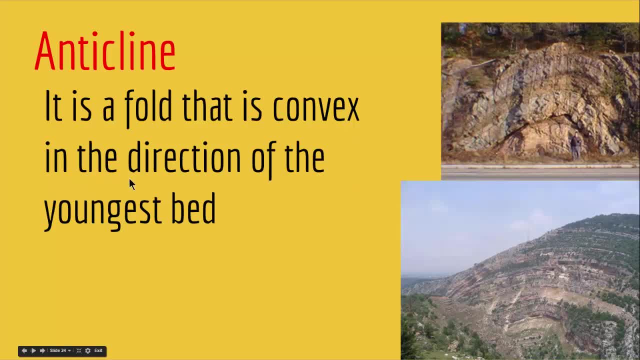 fold them in a way where it's convex in the direction of the youngest bit, just like you see in this picture. it's convex in the direction of the youngest bit. then you get an anticline. Anticlines are an upside down U-shape where the folding is in the direction of the youngest bit. 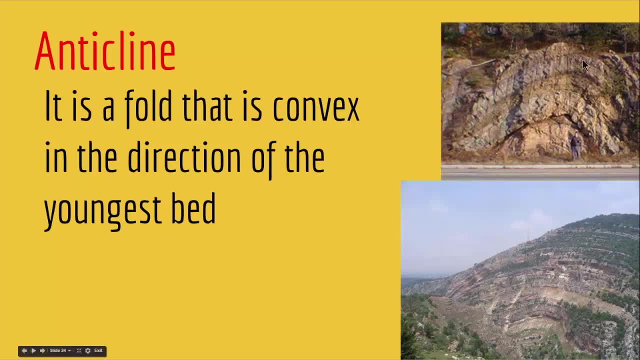 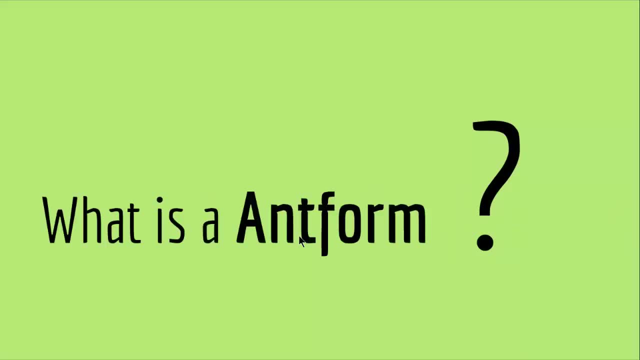 But what happens if you don't know if the layer on top is the youngest bit or the oldest bit? Well, in that case there is another term that is called an antiform. So what is an antiform? Well, an antiform is a fold that is convex upward It is convex. 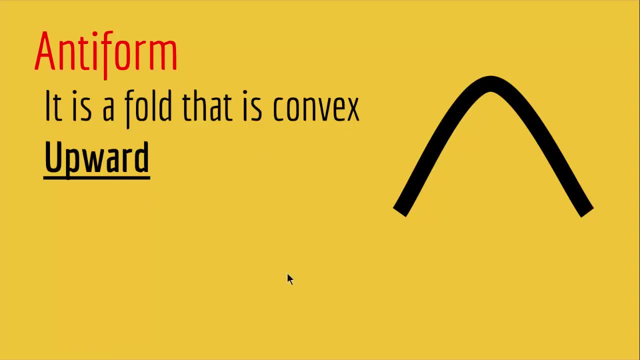 upward. but in case whether you don't know if the layer on top is the youngest layer or the oldest layer, in that case you call your structure an antiform, You do not call it an anticline, you call it an antiform. So antiforms is a fold that is convex upward and anticline is a fold. 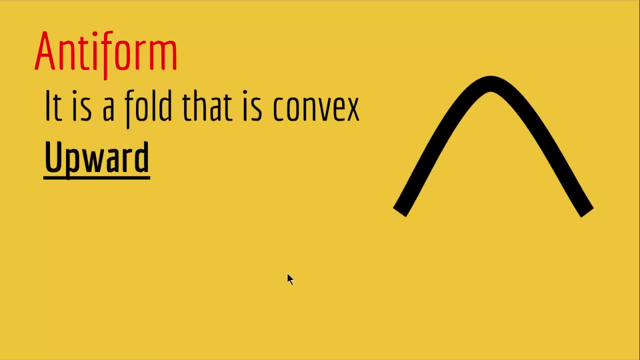 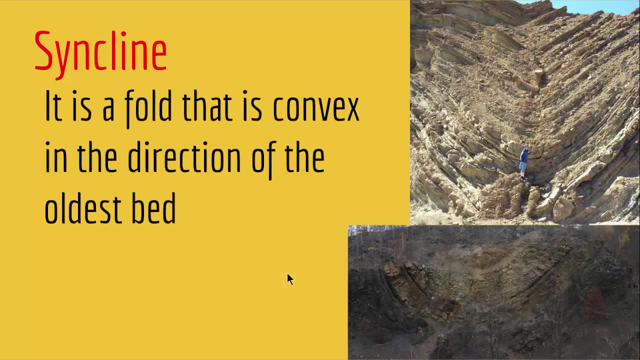 that is convex toward the youngest bit. Another type of folding that we have is called scenicline. So what is a scenicline? Well, a scenicline is a fold that is convex in the direction of the oldest bit. Just like you see here, our oldest bit lays in the ground. 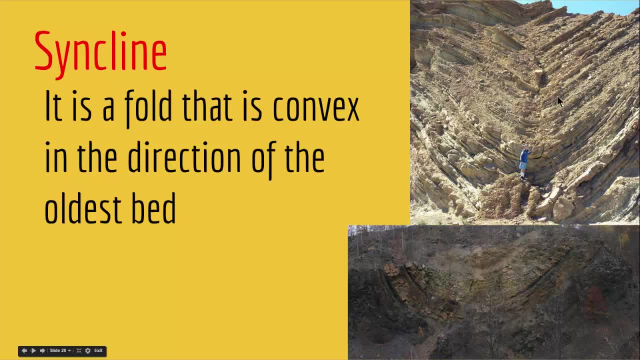 and since we have a convex that is, in the direction of the oldest bit, then we have a scenicline. You have to keep in mind that if, for some reason, this structure gets overturned, your youngest bit will be at the bottom and your oldest bit will go on top. In that case, 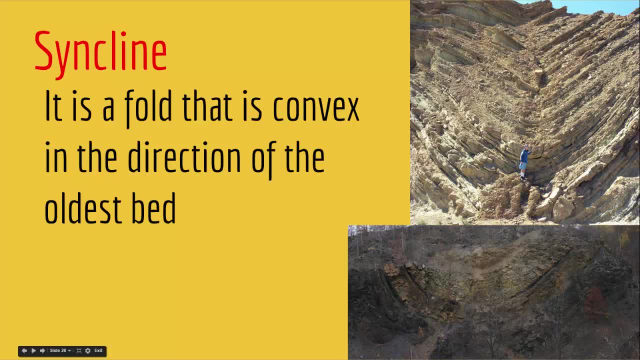 you still have a scenicline, even though the shape looks like an anticline or an antiform, Since you have a convex that is in the direction of the oldest bit. you have a scenicline, just like you see in this picture, But if you don't know whether the convex is in the direction, 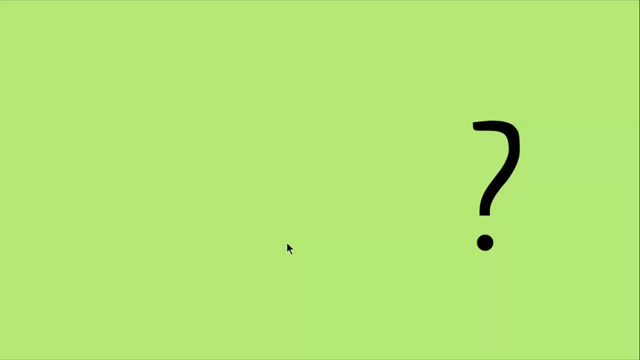 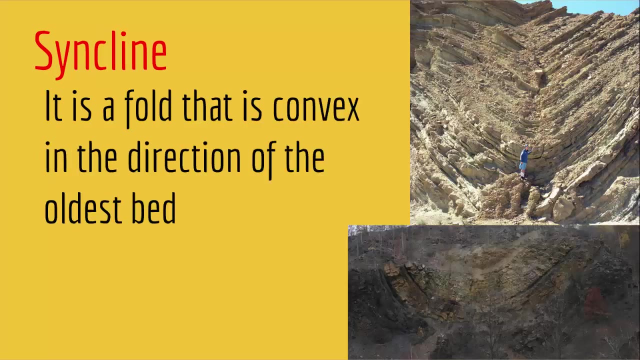 of the oldest bit or the youngest bit. in that case we call it a sceniform. So a sceniform is a fold that is convex in the direction of the oldest bit. So a sceniform is a fold that is concave upward. So sceniclines are convex in the direction of the oldest bit and they are a U-like. 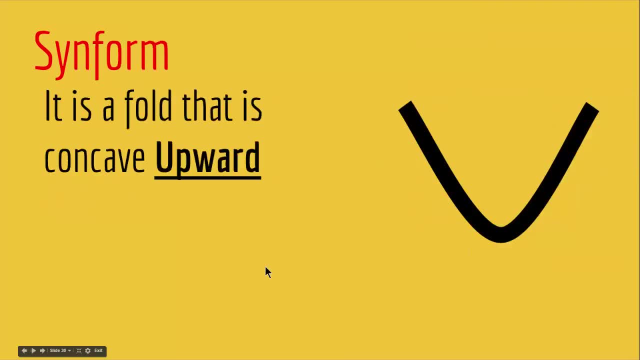 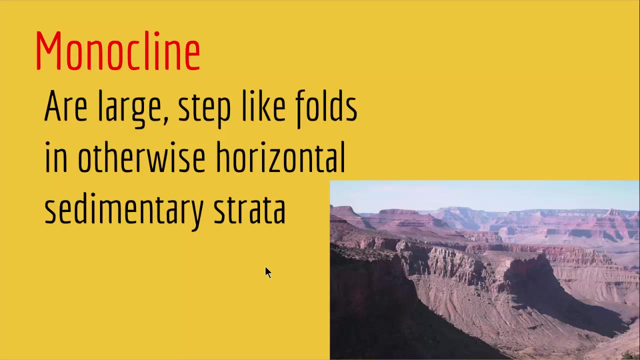 shape, but sceniforms are folds that are concave upward, in case you don't know whether your oldest layer is on top or in the bottom. Another type of folding that we have is called a monocline. So what is a monocline? Well, monoclines are large step-like folds in otherwise, 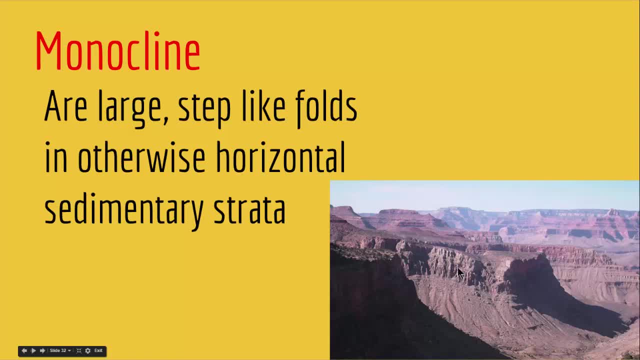 horizontal sedimentary stratas. Monoclines are not U-shaped, whether they are U-shaped upward or downward, but actually they are step-like. So you have a horizontal layer and then you have an inclination and then you have another horizontal layer. So it goes like this: it bends and it goes flat again. Those are called monoclines. 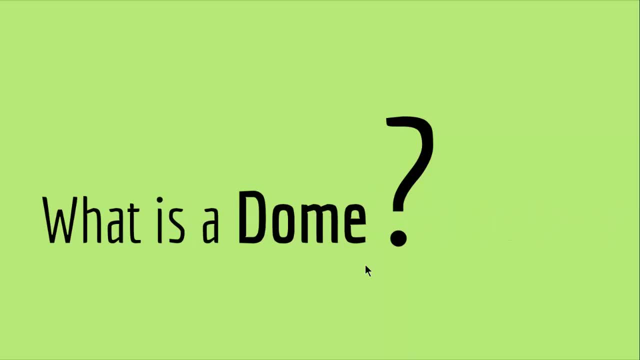 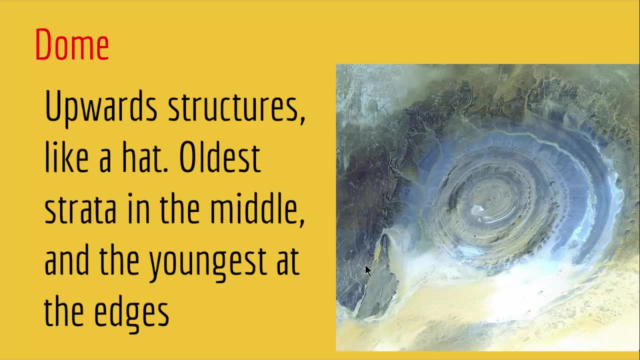 Another type of folding that we have is called a dome. So what is a dome? Well, a dome is an upwards structure like a hat, where the oldest strata is in the middle and the youngest at the edges. Imagine you have stratas of rock and these stratas bend upwards and they create a hat-like. 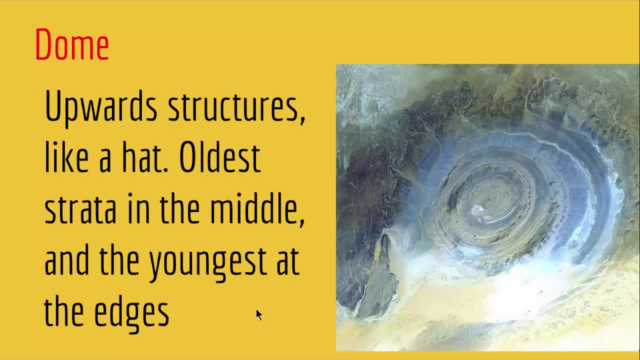 shape where the oldest strata is in the middle and the youngest is at the edges, Just like you see in this picture. you had stratas and for some reason, all of them went in an upward direction. They created a hat-like structure where your oldest strata is in the middle. this is the oldest. 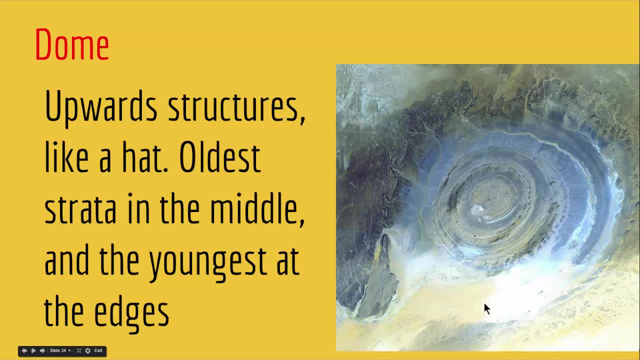 and the youngest is at the top. These are called domes because they resemble a dome, But, as you can see, all the layers have been eroded away and the vertical stratas have been exposed. The exact opposite of domes are something that is. 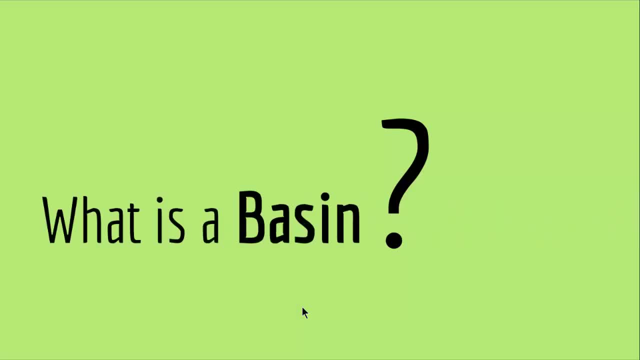 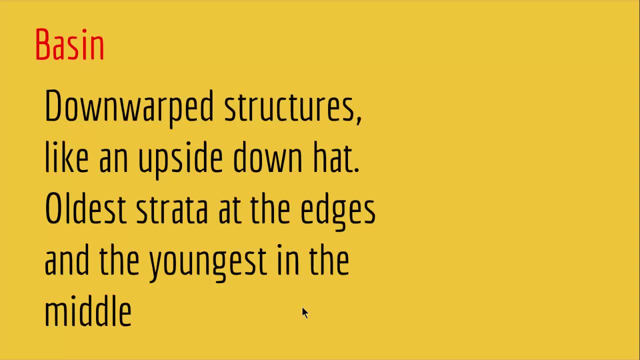 called basins. So what are basins, or what's a basin? Well, a basin is a downward structure, like an upside-down hat, where the oldest strata is at the edges and the youngest is in the middle. So imagine you have rock stratas and for some reason, these rock stratas